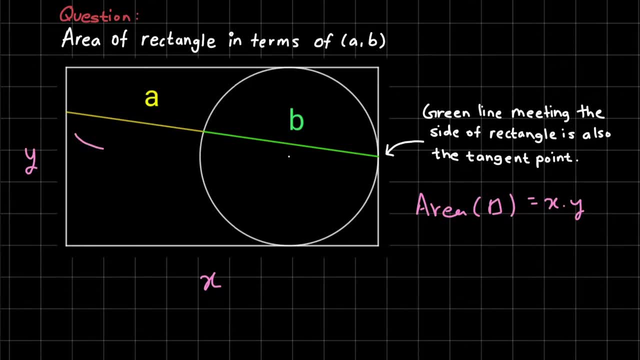 this rectangle and that is the main thing that is defining the position of this particular line segment. so the first thing that i can notice is that this particular circle is tangent at this, this and this three points. so i will simply draw the radius to all these three points. 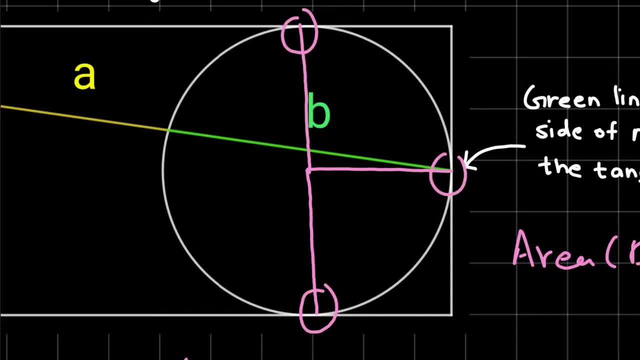 now, these are the three points where i have drawn the radius, and all these three points are tangent points. now we all know this theorem very well, that is, the angle form at the point of contact between the radius and the tangent line is always 90 degree. so because of this particular 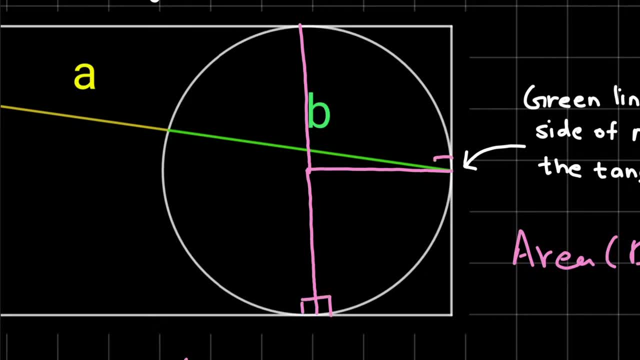 particular theorem: this angle over here would become 90 degree, this angle over there 90 degree and this angle would also be 90 degree. Now, this angle and this angle would also be 90 degree, because these two angles are ultimately the corner of a right triangle. 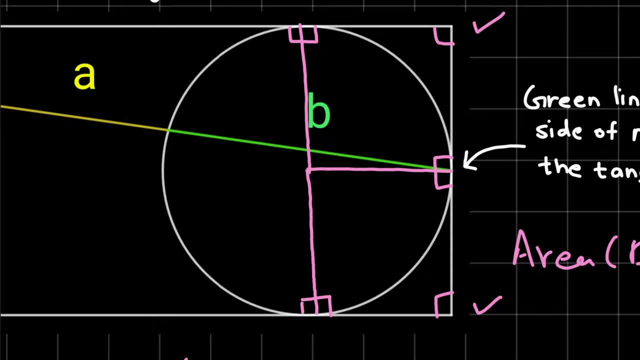 and in right triangle, all the corner angles have a value 90 degree. Now we have two quadrilaterals over here. one is over here and the other one is over here. In both of them, we can clearly see that three of the angles have a value 90 degree. Therefore, by applying the angle, 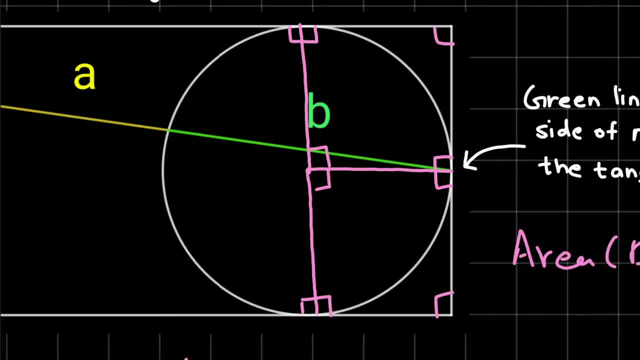 sum property, the value of the fourth angle would also be 90 degree. Now, as we can see, this point is common. between this and this line segment that is the center of the circle, and the addition of this and this angle completely forms 180 degree. This ultimately shows that: 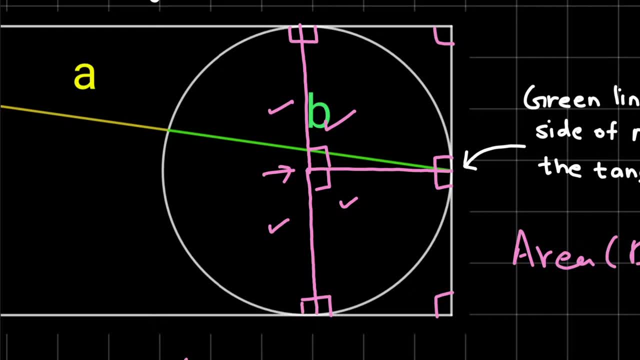 this particular line is a straight line. In other words, we can say that this point, the center of this circle, and this tangent point are collinear points. ok, Now let me just clear this thing and we will go forward in the solution. Now, what if I take the radius? 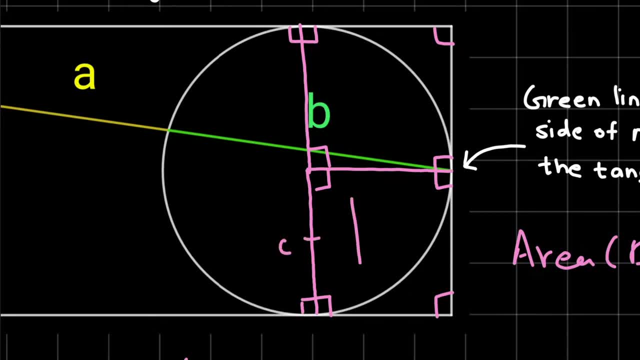 of this circle, something like c. so we can see that this particular quadrilateral over here is a square. why? because all the four angles are 90 degree and these two adjacent sides are equal and they are ultimately the radius of the circle. similarly, this quadrilateral is also a square because all the four angles are 90 degree. 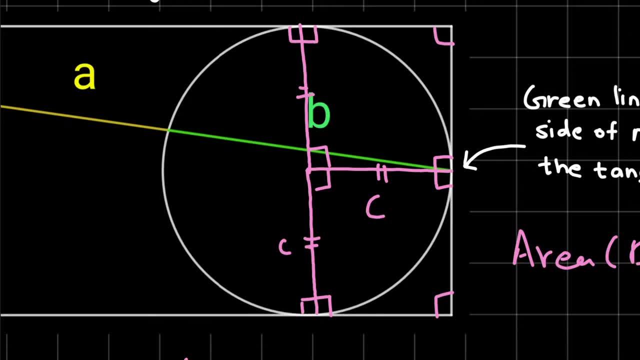 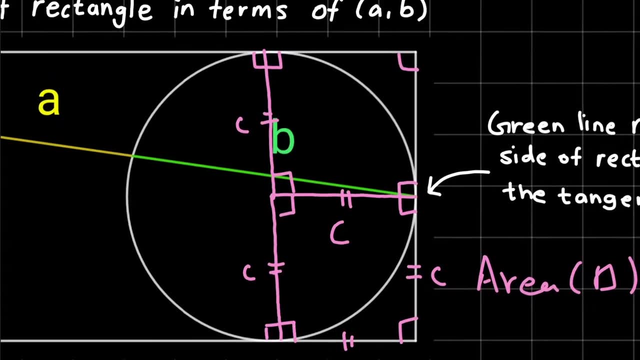 and adjacent sides are equal and they are ultimately the radius of the circle. so in a square, all the four sides are equal. so this length would also become c. this length would also be equals to c. this length would also be equals to c and this length would also be equals to c. now what i can. 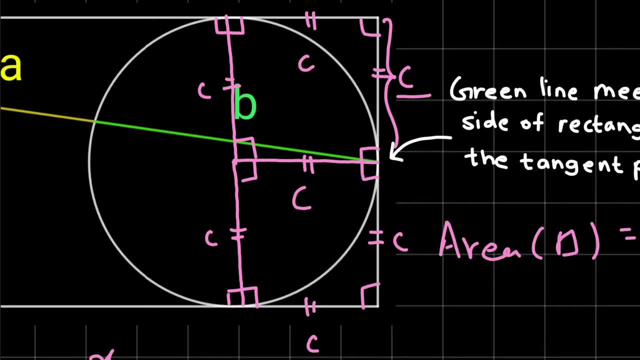 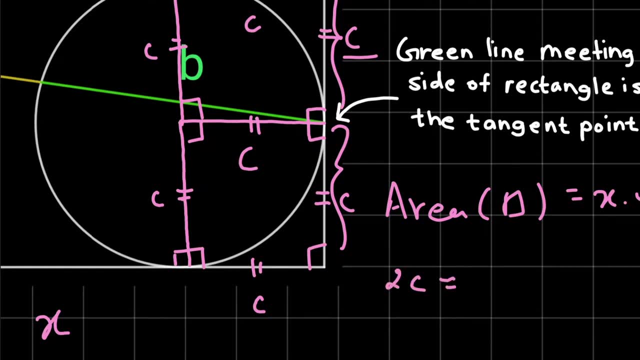 say is that the length from here to here is equals to c and the length from here to here is again equals to c. so the addition of this bottom will completely form two times c, and that is ultimately the breadth of the rectangle and that we have already taken as a variable y. so two times c. 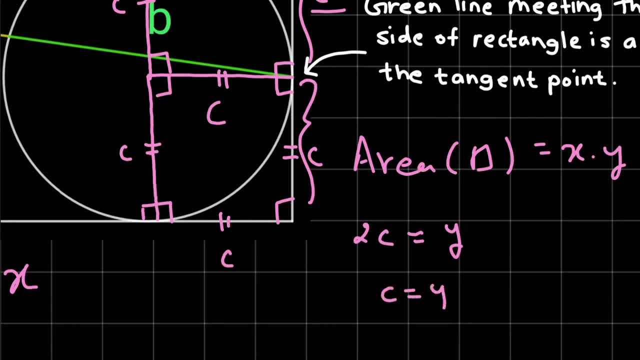 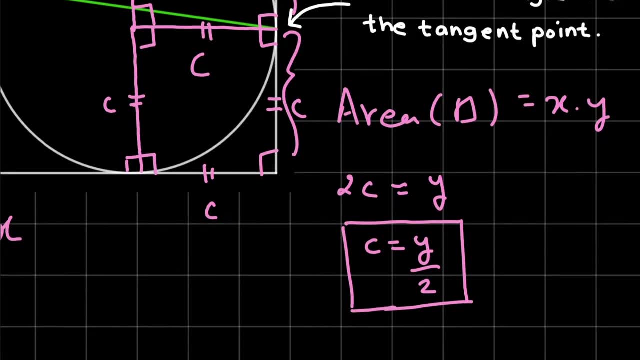 equals to y. solving this equation will get the value of c, and that would be y upon two. so here we have ultimately got the value of radius of the circle in terms of y, and that is y upon 2. so i will just clear all these things and keep only one of the radius that 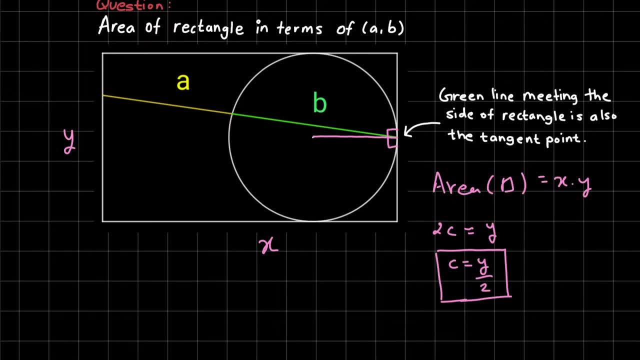 is. so the radius that we are going to keep in this diagram is this particular one. okay, now let me tell you a thing: that there are two solutions to this problem. so first of all, let us see the first method- and this is basically the method i first of all did to find the solution- and the second method i 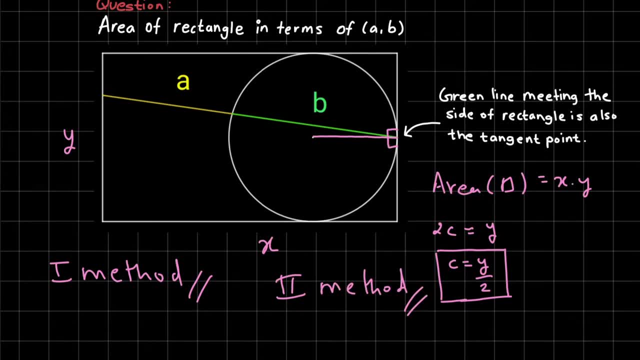 got so the second method. i got in this particular manner, like i have done my first method, and got the answer to this particular problem. now, when i was checking the answer that, whether my answer is correct or not, using the first method, the final answer, i came to know about the second method. 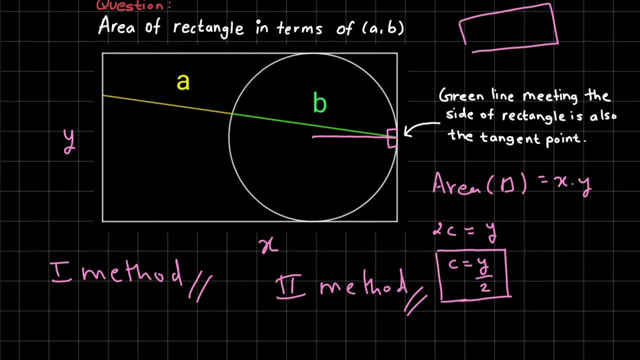 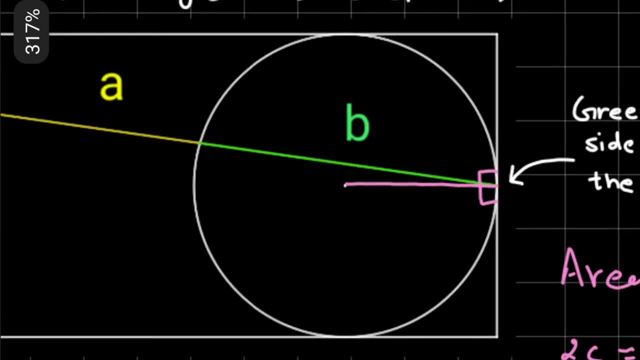 with which they have done in order to get their final answer. so i will be presenting both of the method, but first of all let us see the first method that i did. okay, so i have just left this radius over here, and that is already meeting at 90 degree to the tangent line, because that point 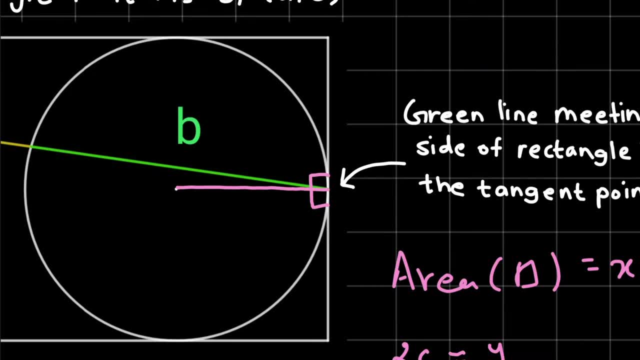 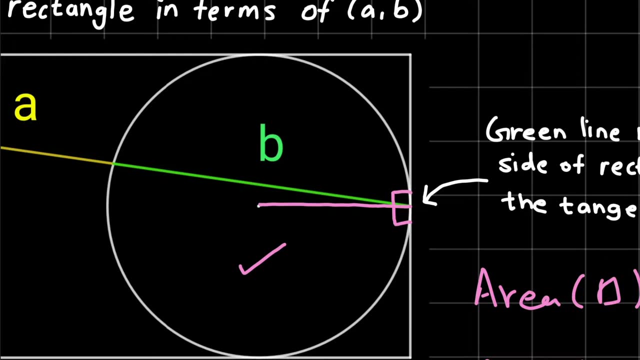 is the tangent point clearly mentioned over here. now, the second thing to be noted in the same statement is that this particular line is also ending at that particular point. take a clear note of this particular thing. okay, now what i will do is i will draw one more radius in this circle, but this time this radius would not. 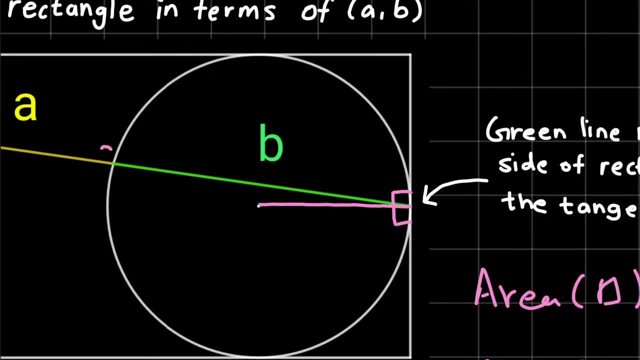 be ending to a tangent point. instead, it will be ending at this particular point where this line segments are getting divided as a and b. so i'm just going to draw the radius like this particular manner. okay, let me do it a bit more clear. so now what we can see is that we have a triangle over 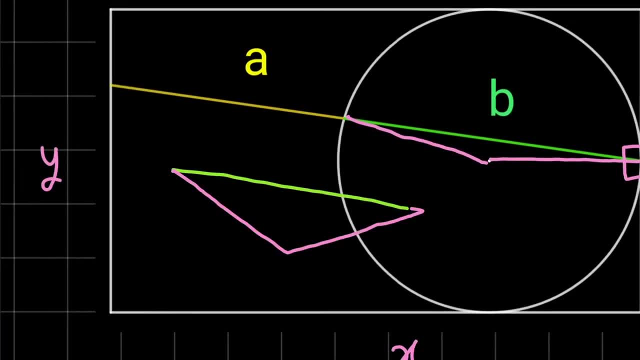 here. let me just redraw this triangle over here and then we will be able to see that this is the triangle in a bigger size- the same triangle. i've just redrawn it over here because that triangle is bit more slimmer, so we cannot explain anything inside. okay, so this length is equals to b and. 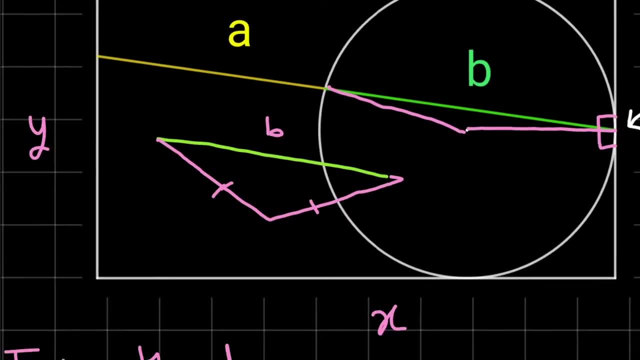 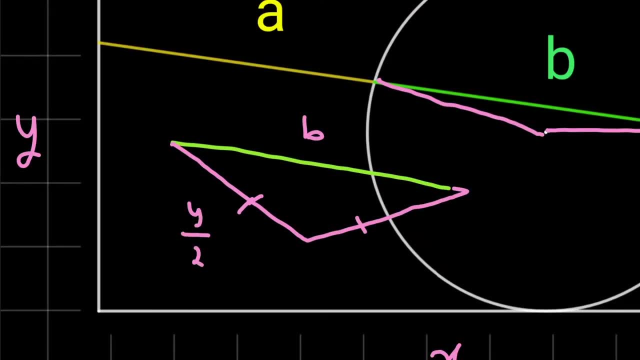 these two are ultimately the radius of the circle, and recall that we have just now got the radius of the circle in terms of y, and that is y upon 2, so both of this length would have a value y by 2. okay, now, what i will do is i will simply mark an angle inside this, so i will simply take this angle as 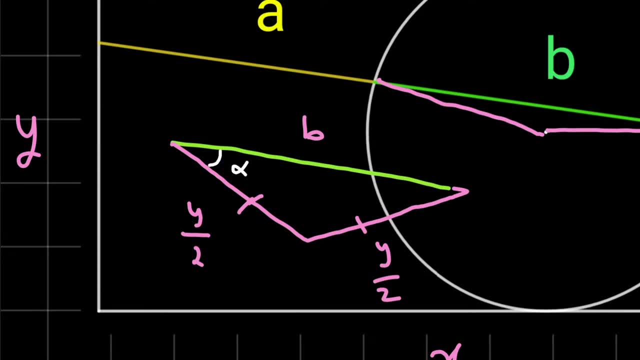 equals to alpha. now look carefully. this triangle is not going to be the same as the previous one, so i will just take this angle as equal to alpha, and then i will simply take this angle as equal to alpha. now look carefully. this angle is an isosceles triangle. these two sides are equal. so if that angle has a value alpha, this: 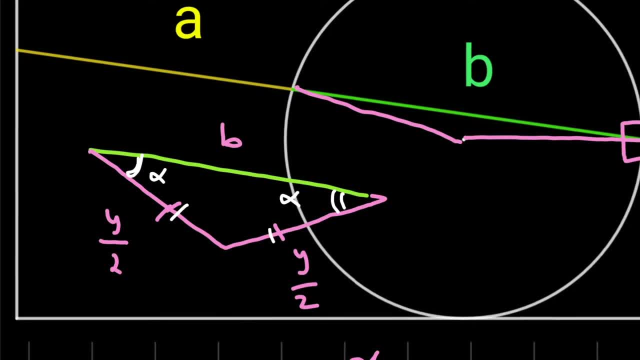 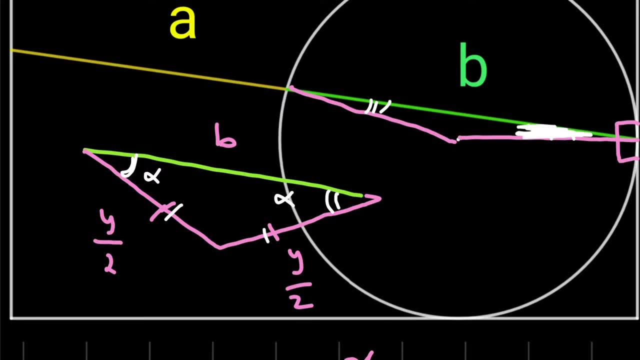 angle over here would also have a value alpha, and in this diagram this angle would be equals to alpha and this angle would be equals to alpha. now look carefully. this much angle is equals to alpha. this complete angle is 90 degree, so the remaining angle would simply be 90 minus self. i will just explain. 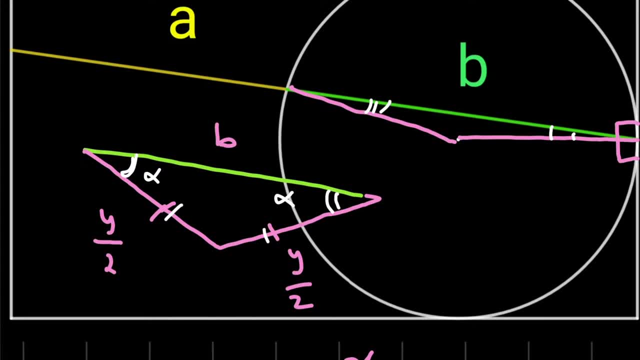 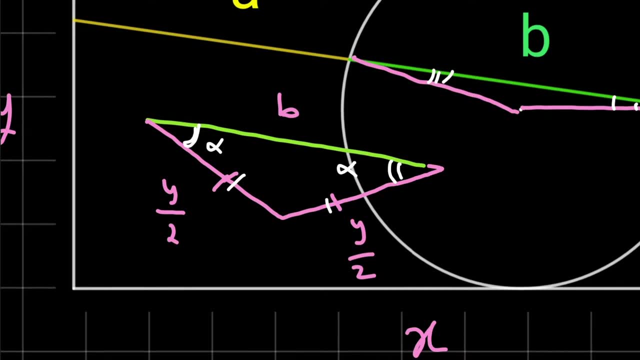 that thing a bit more later, when it is required. just now, concentrate on this particular triangle in which we have two angles as alpha and alpha, and all the three sides are y by 2, y by 2 and b. so now what we are going to use is the cosine rule. so, simply, the cosine rule is like this way, if you, 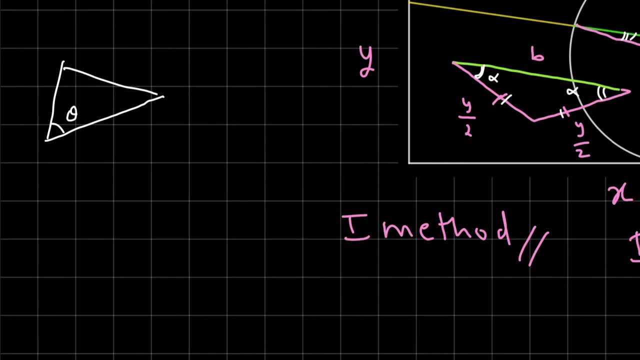 have a triangle. in this triangle, if you have one of the angle as theta and the three sides are a, b and c, then the value of cos of theta would be equals to squares of the adjacent added together. so adjacent to angle, theta are a and b, so a square plus b square minus the square of opposite. so 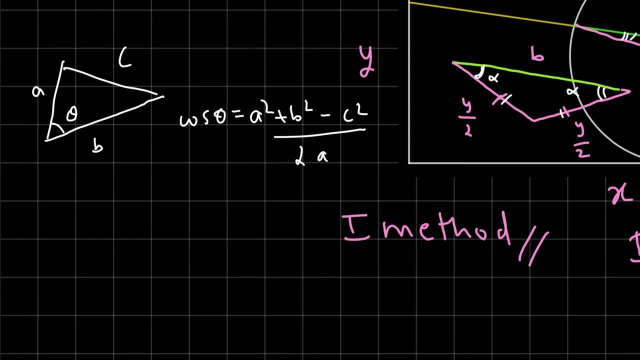 minus c square upon two times the product of adjacent, so two times a times b. this is the value of cos, of theta, in a triangle with sides a, b, c, using the cosine rule. so this is the cosine rule we are going to use over here in this triangle. so we have the angle alpha. so i will take that only. 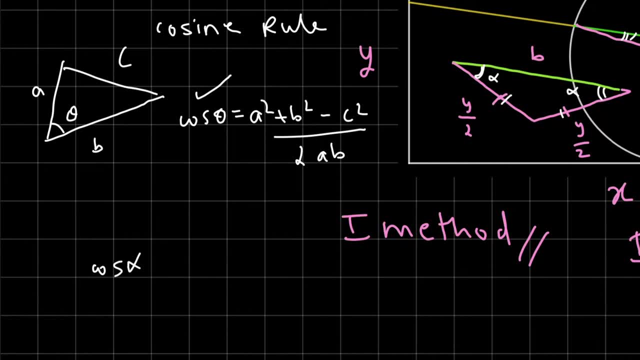 so value of cos of alpha in this triangle would be squares of the adjacent added together, so adjacent side to this particular angle, alpha. you can take any of them, you will get the same result. so i am just going with this one. so the adjacent sides are y by 2 and b, therefore y upon 2. the 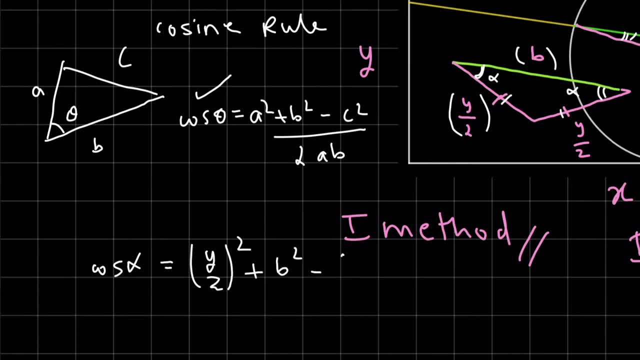 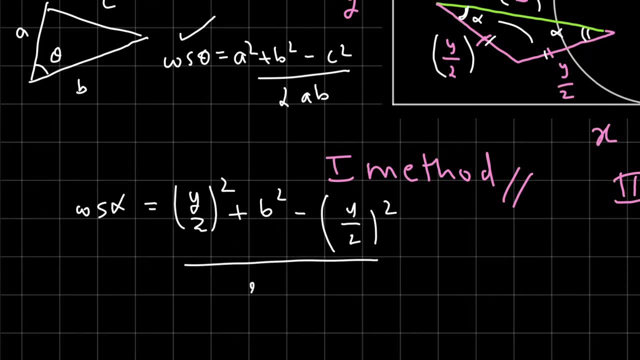 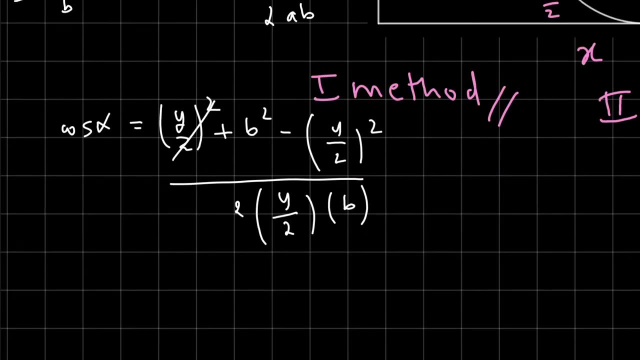 complete square plus b square minus the square of opposite, so opposite to angle. alpha is equal to b, so the cosine of alpha is again y by 2, so minus y upon 2, the complete square divided by 2 times the product of adjacent, so 2 times y by 2 times b. now in the numerator we can clearly see that these two 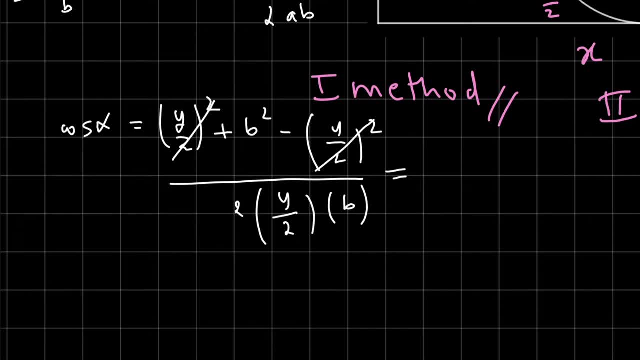 will cancel out each other. we will finally left with b square upon this thing. the b will cancel out the b square. so finally, the value of cos of alpha will turn out to be b upon. now look carefully this 2 and 2 is also going to cancel. so b upon y is the final value for cos of alpha. this is an. 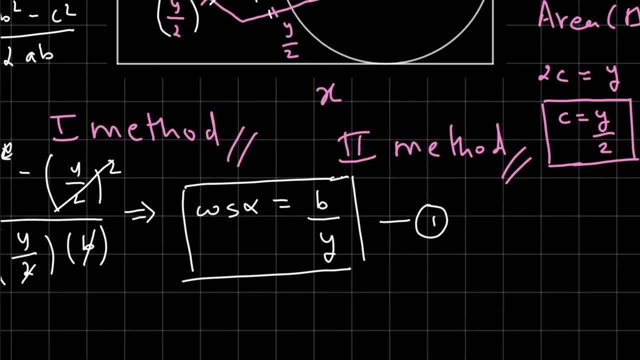 important result, so let it be done. so this is the final value for cos of alpha. so this is the final value for cos of alpha. this is an important result, so let it be done. equation number one: okay, the second method we will see later on, so let it remove that. 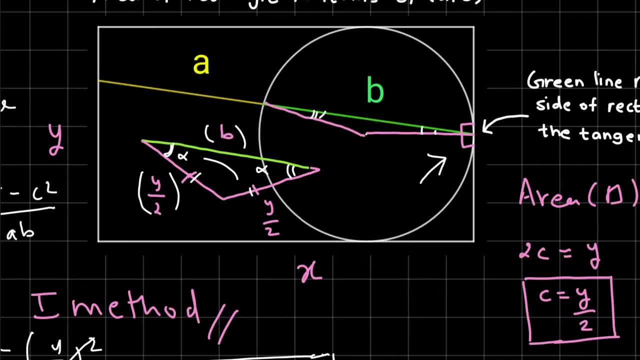 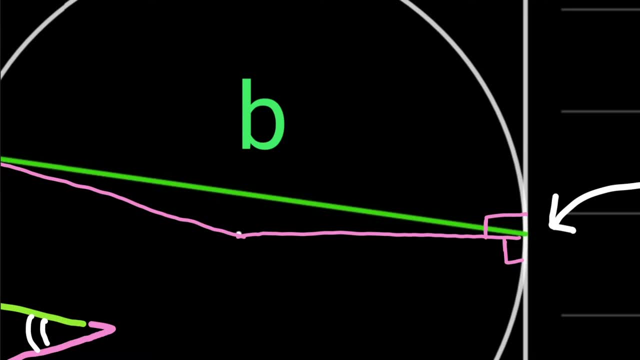 now let us see this particular thing that i was saying. we have to subtract the angle alpha and all that thing, so i have to just zoom over there, okay. so here i have just redrawn everything, but in a clear manner. now let us mark the angles alpha. so the angles alpha were this angle and 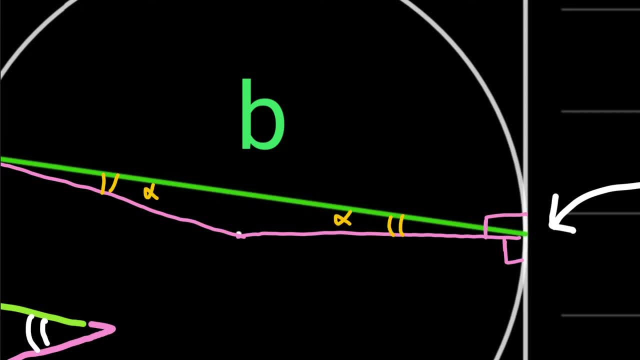 this angle and they were having a value alpha. okay, now what i can see is that the angle between this particular white line and this radius, that is, the pink line, is already 90 degree. okay, now, the angle between this pink line and this green line is equals to alpha. therefore, the remaining 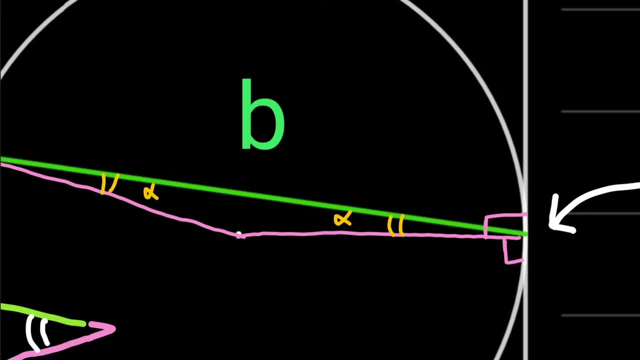 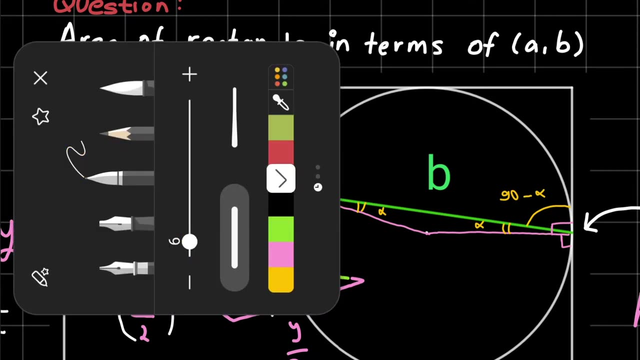 angle that is between the green line and this white line would simply be 90 degrees minus the alpha. so this angle between the green line and the white line would have a value 90 minus alpha. okay, now what i will do is i will just construct one more line segment, and this will be from this particular 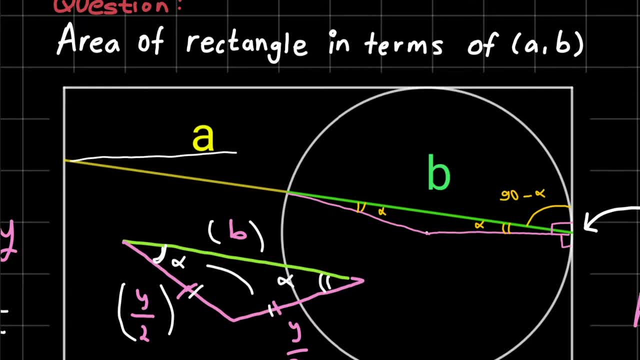 point where the line segment is getting started, from this point to the right side of this rectangle. okay, now look carefully that this angle is 90 degree because it is the corner of this right triangle. this angle is also 90 degree because it is the corner of the rectangle. this is 90 because that. 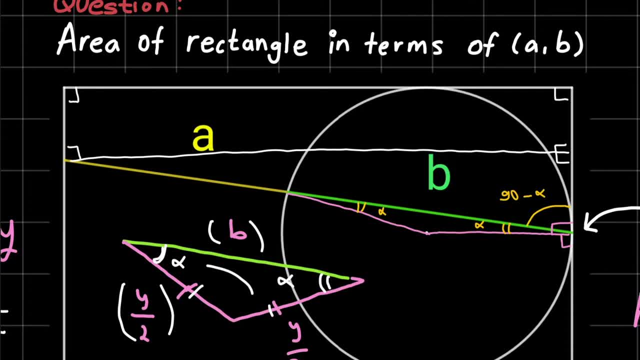 we have constructed, and therefore by angles and property. this is also 90 degree, this white line and this white line. okay, now, as all the four angles are 90 degree, this particular quadrilateral becomes a rectangle. now, recall that the length of this biggest rectangle, we have already taken it as 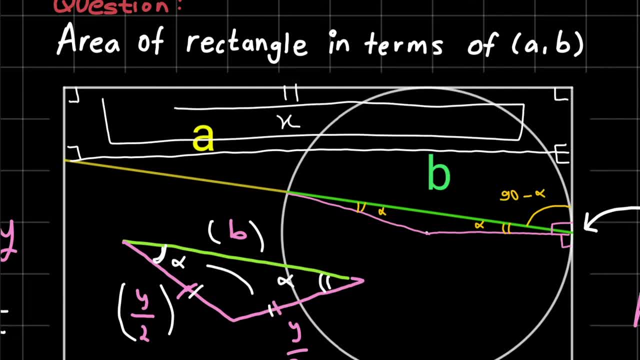 a variable x. hence, when this particular quadrilateral becomes rectangle, this length would be equals to this length that is already having a value x. therefore, the length of this white line segment would also be equals to x. okay, so i'll just remove this thing. so keep this thing in mind. this complete white 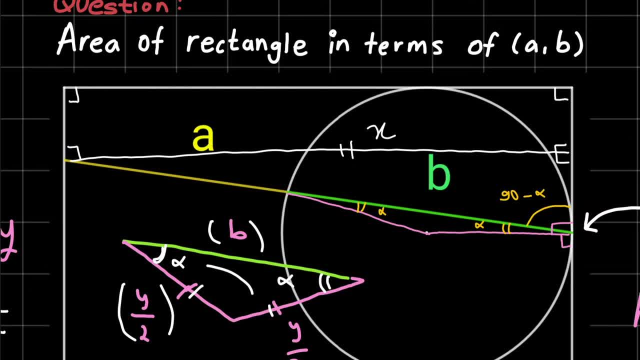 line segment is having a length x. okay, now look carefully in this particular triangle that is ultimately a right angle triangle. let me just label this thing. so let this point be p, this point be q and this point be r. so look in this right angle triangle, pqr, it is right angle at the point. 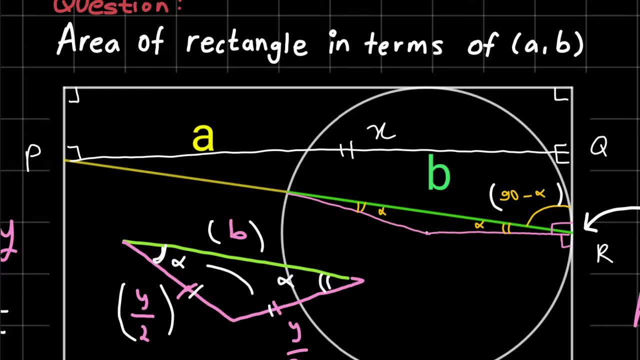 q, the other angle at the point q and this point b q and this point b r. so now let me just label these things. angle is having a value 90 minus alpha. so in this triangle, two of the angles are 90 and 90 minus alpha. therefore, by applying the anglesome property, the value of this third angle would simply be: 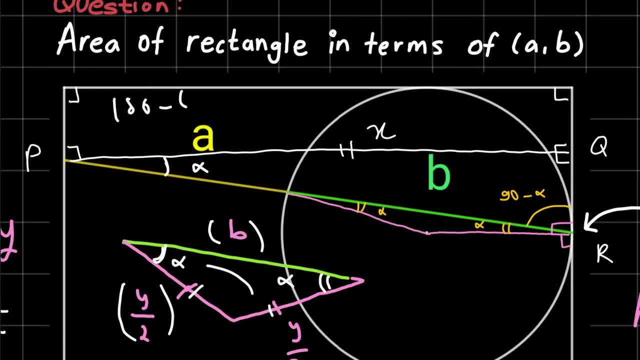 alpha. you can apply the anglesome property 180 degrees minus 90 plus 90 minus alpha. so this thing will result in alpha and that would ultimately be the third angle. so in this right angle, so in this right angle triangle pqr, we can see that one of the angle is alpha. so from the 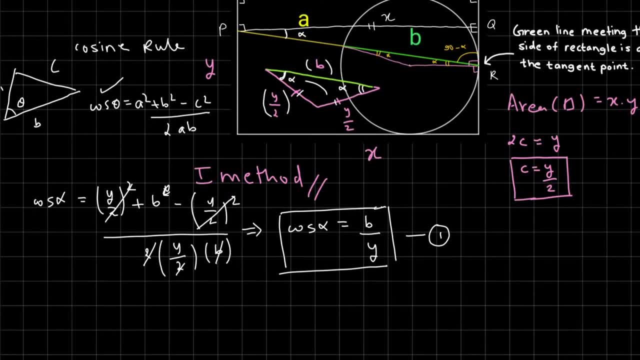 perspective of this right angle triangle. so let me write it down. so from the perspective of that right angle triangle, that is, the triangle pqr, the value of cos of alpha would simply be based upon the hypotenuse. base is the complete white line, that is, having a value x upon the hypotenuse. so 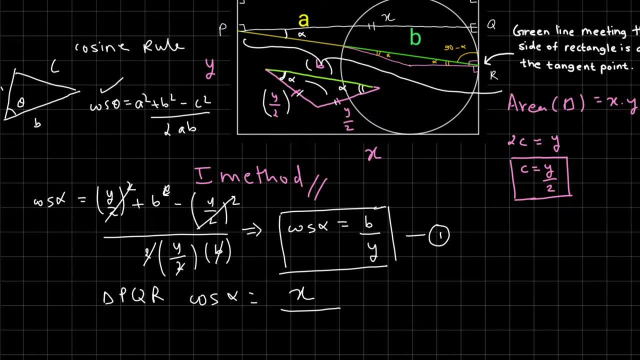 the hypotenuse is from the point p to the point r, and that is ultimately a plus b. this complete length is ultimately the hypotenuse for this right angle triangle. so ultimately, from this right angle triangle, pqr, we have got the value of cos of alpha. so from this right angle triangle, pqr, we have got the value of cos of alpha. so 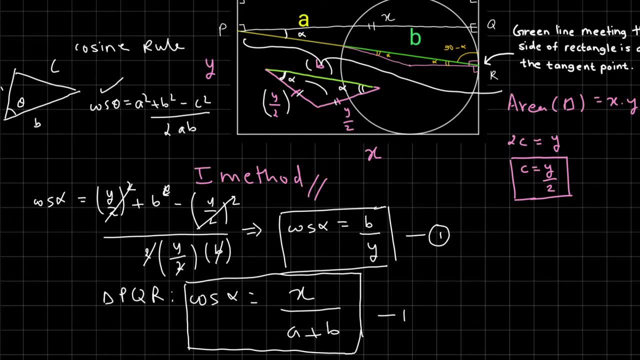 that is, x upon a plus b. now look carefully in the first equation and in the second equation. we can clearly see that both of this equation give us the value for cos of alpha. hence we can compare these values. therefore, b upon y, that is, this thing, would be equals to this thing, that is. 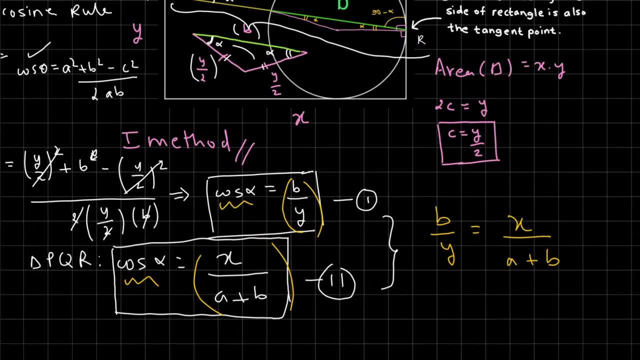 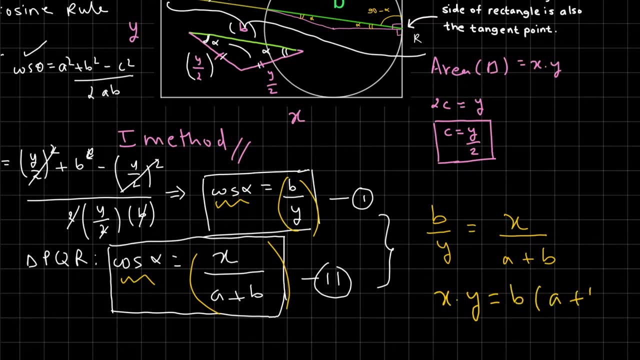 going to be x upon a plus b, and if i will simply do the cross multiplication, i will get x times y equals to b times a plus b, and this is the answer that we are ultimately looking for. look carefully, we have got the value for x times y and that is ultimately representing the area of the right triangle and the question. 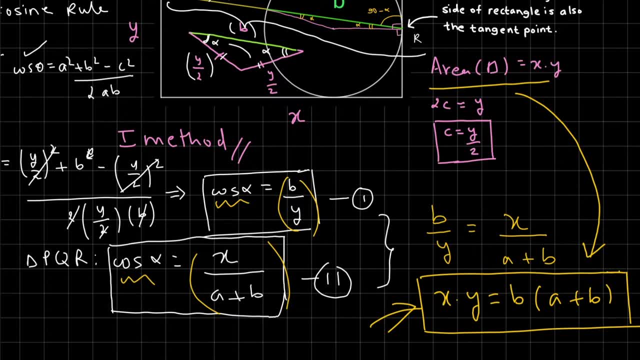 was to find the area of the right triangle in terms of a and b, and that we have done. the area of the right triangle has been found completely in terms of a and b. okay, now, this was the first method. now let us see the second method, and i think the second method is more simpler than this. 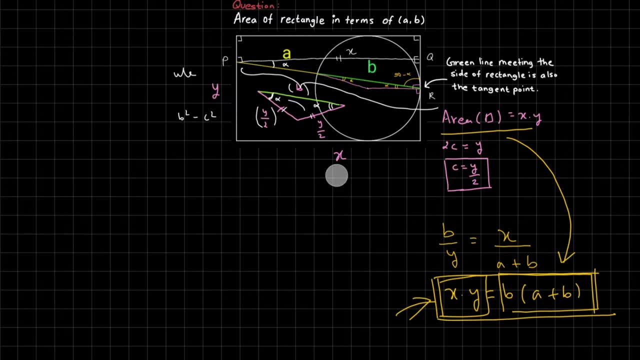 one. this is the first method that i thought so that is necessary to be presented now the second method for your convenience. so i am just removing all these things. i'll still keep this thing that yes, this is the length and this is the breadth that i have taken. 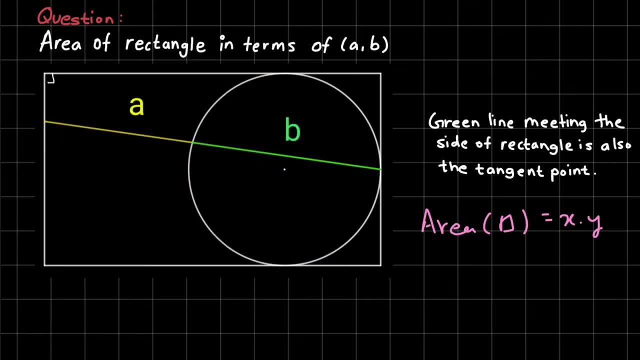 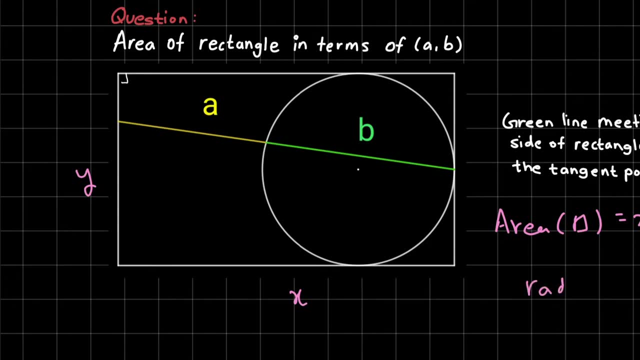